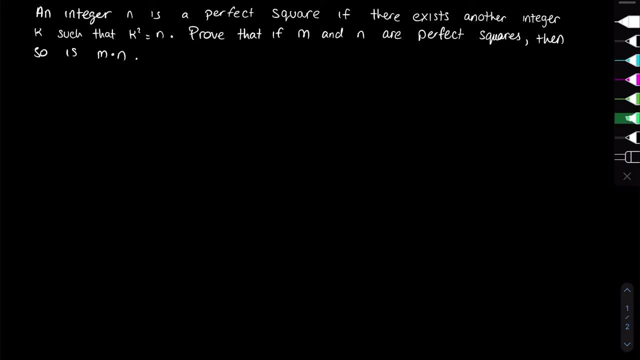 assign another name for n times n, so we don't have to write n times n every time in our proof. So let's say: let z equals to m times n, And let's start proving it now. So suppose m and n are perfect squares. Then by the definition they give us, which is on the first line, 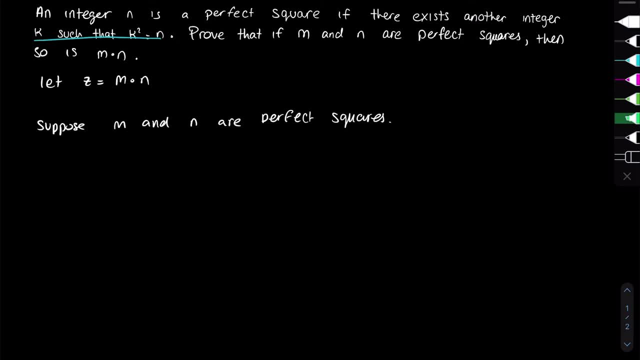 we know that there must exist a, an l. An l is an integer, a random integer, We don't know which integer, But there exists an l, And if you square that l, we get m, since m is a perfect square. And likewise there. 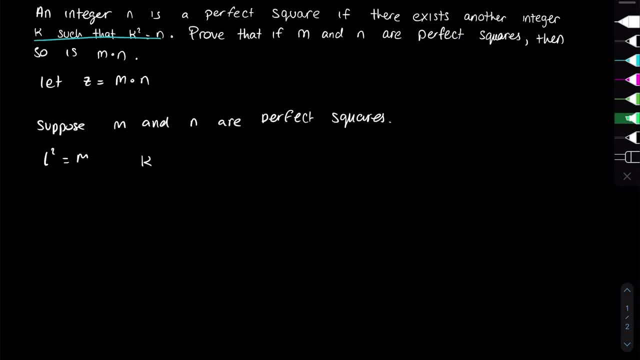 exists a k. k is also an integer. We don't know what integer it is, But if we square it, then we get n. Now we want to prove that, since m and n are perfect integers, we want to prove that z is also a perfect integer. 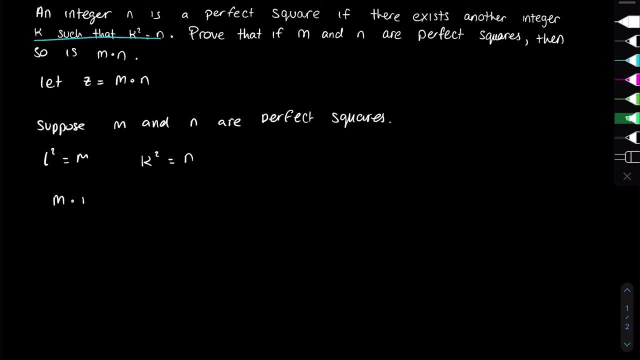 So let's start off by saying m times n, And this according to what we found out right here on the previous line. we can substitute m by l squared and n by k squared, So now we have l squared times k squared, So we have a number squared times another number squared. 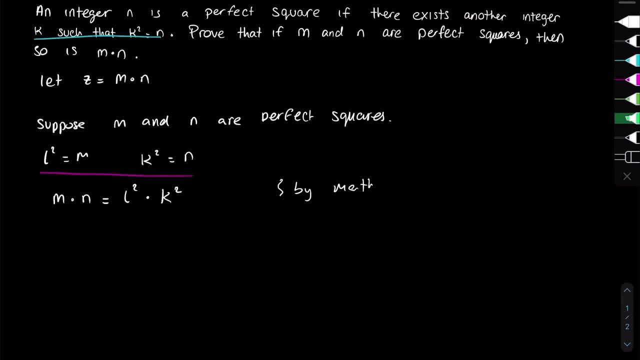 And by mathematics we know that this is the same as l times k all squared. This is just a rule. Now we also know that m times n. we call it zed. so we just call it zed because we don't want. 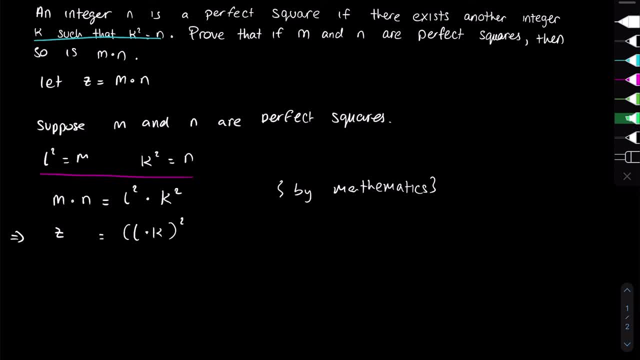 to write m and n times n all the time, And now there isn't much else to do anymore because realistically, we've already proven that zed is also a good integer, And so now we can prove that. we've already proved that zed is also a good integer, And now we can prove. 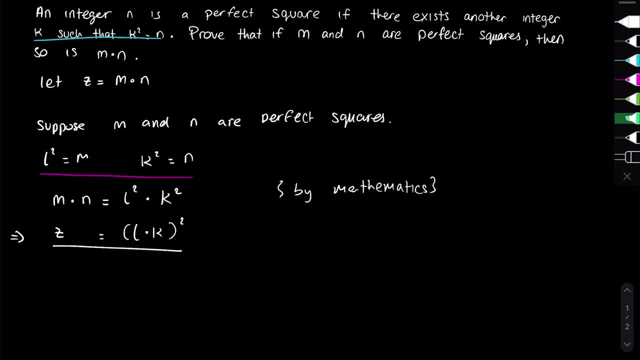 that m and n are perfect integers, And so we know that zed is also a good integer And a perfect square. How you might ask? Well, the definition of a perfect square states if there exists an integer k and if you square it, then it gives you n or z or m in this case. Well,